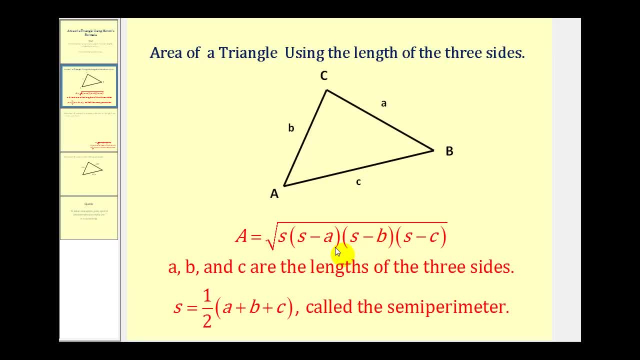 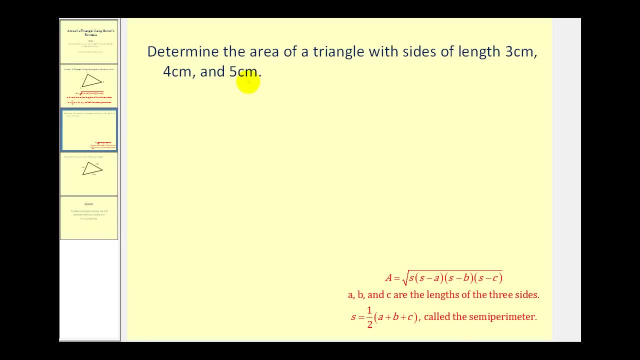 how to apply this formula. Let's go and take a look at our first example. Here we want to determine the area of a triangle with sides of length 3 centimeters, 4 centimeters and 5 centimeters. So the area is going to equal the square root of s times s minus a times s minus b. 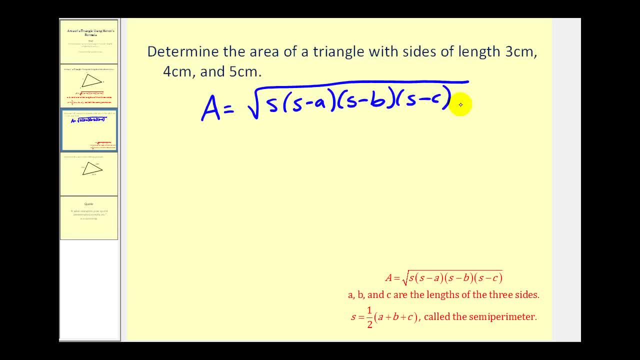 times s minus c. So let's go ahead and let a equal 3,, b equal 4, and c equal 5.. Remember, s is the semi-perimeter, or half of the perimeter. So let's go ahead and find the value of s. It's going to be one half times the quantity. 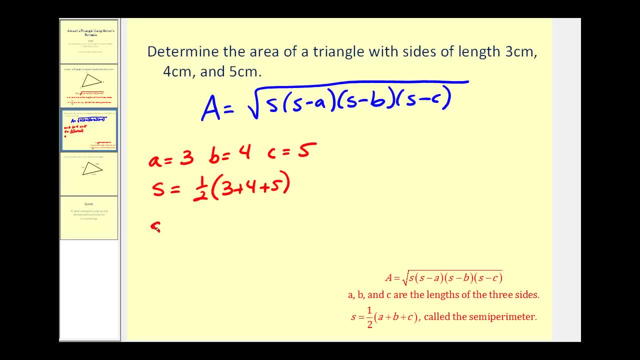 3 plus 4 plus 5.. That's going to give us 1 half times 12.. So s is equal to 6.. So now we can go ahead and apply the formula: Replace s with 6,, a with 3,, b with 4, and. 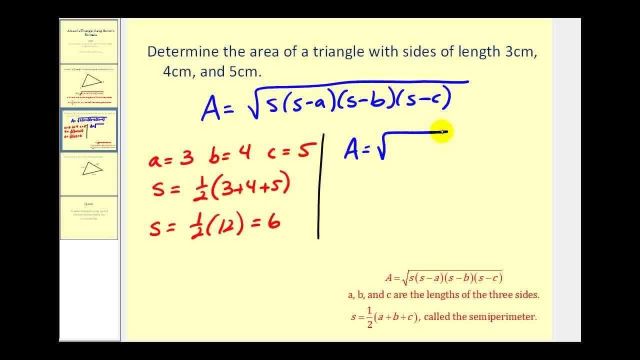 c with 5.. So we're going to have the square root of 6 times 6 minus 3, times 6 minus 4, times 6 minus 5.. Let's go ahead and simplify this. We're going to have 6 times 3 times 2 times 1.. This is going to be: 6 times 3 is 18, times 2 is 36,. the 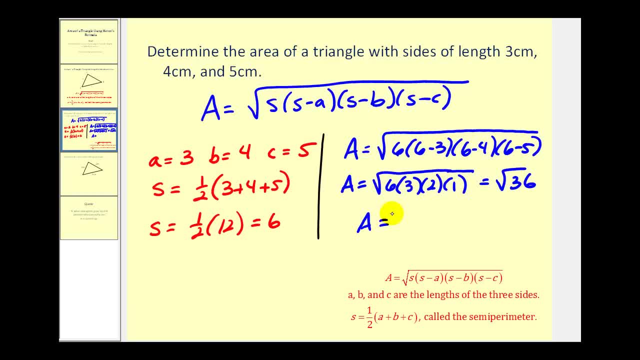 square root of 36.. So the area of this triangle with sides length 3,, 4,, 5 centimeters is equal to six centimeters squared. Now, I'm not sure if you recognize this, but a triangle with sides length three, four, five. 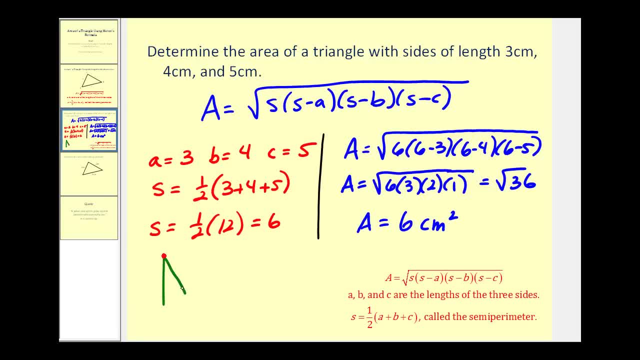 is a right triangle where the shortest leg would be three, the longest side would be five, the hypotenuse and in this case the height would be four. So, using the traditional area formula for a triangle, area equals 1 1⁄2 base times height. 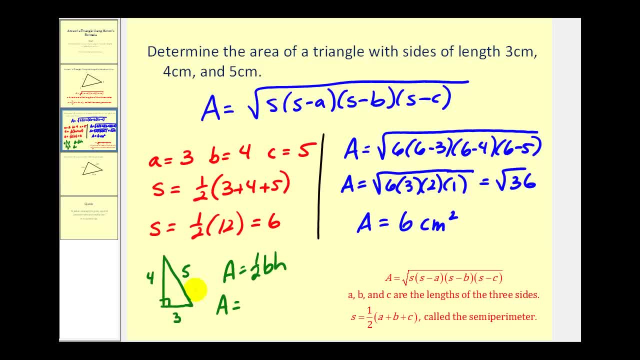 we could verify the area that we found using Heron's formula. It'd be 1 1⁄2, three times four, which of course is also six. Now remember to use this formula here. we do have to find the height of the triangle. 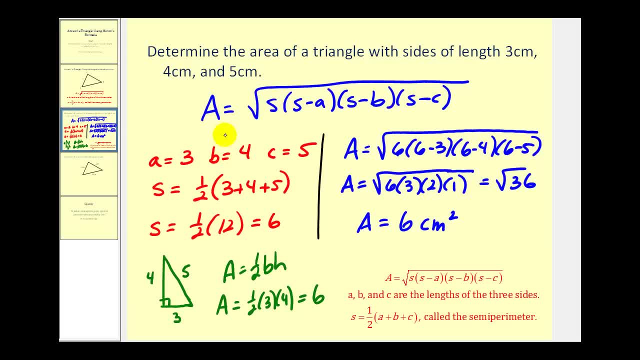 and we lucked out here because it was a right triangle. but what's special about Heron's formula is we don't have to have the height and it doesn't have to be a right triangle, We just have to know the length of the three sides. 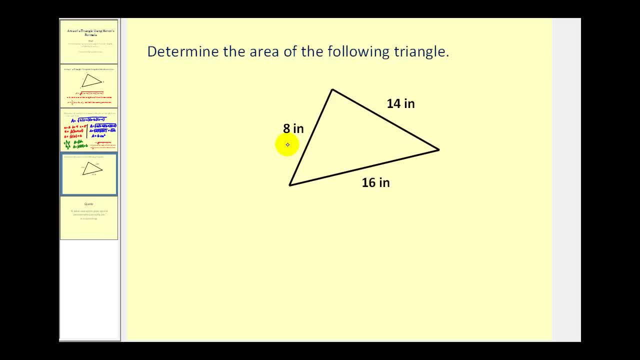 Let's go and take a look at one more example. Here we have a triangle with sides of length eight, 14, and 16 inches. Just to keep things organized, let's go ahead and call this A. We'll call this B. 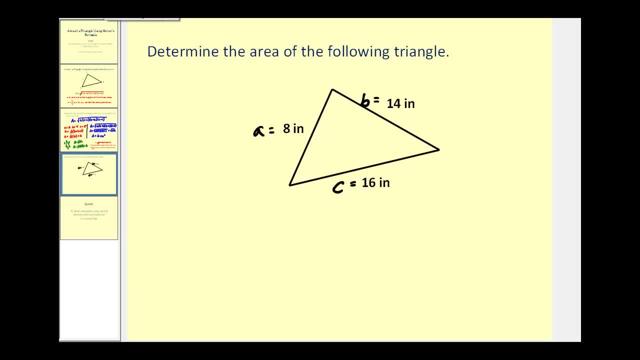 We'll call this C. Let's go ahead and write out Heron's formula. The area is going to equal the square root of S, times S minus A, times S minus B, times S minus C. Let's go ahead and determine the value of S. 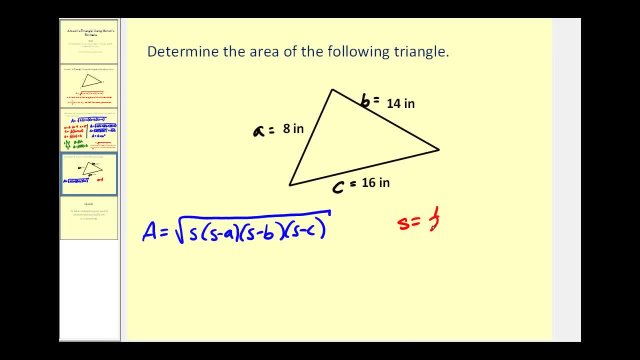 which is half of the perimeter. We're going to have 1⁄2 times the quantity of eight plus 14 plus 16.. It's going to give us 1⁄2 times. looks like we'd have this would be 30 plus eight. 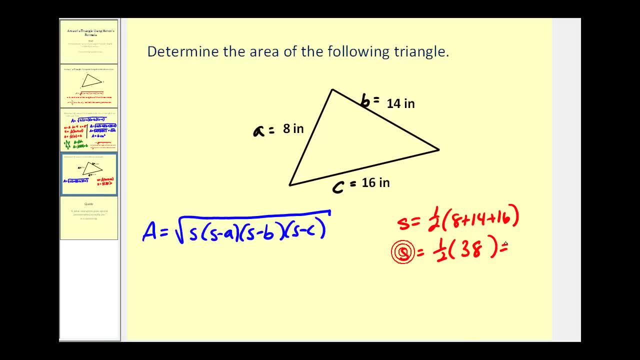 so we have 1⁄2 times 38, so our semi-perimeter is equal to 19.. Let's go ahead and apply our formula. The area of this triangle is going to be equal to the square root of 19 times 19 minus A, which is eight. 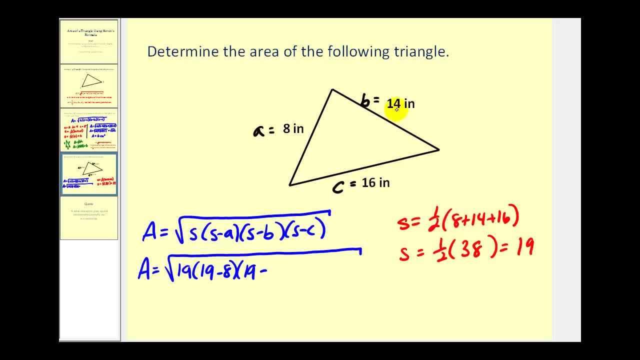 so 19 minus eight times 19 minus B, so 19 minus 14, and then, lastly, we have 19 minus C, and then C is 16.. Let's go ahead and simplify this. We have 19 times 11.